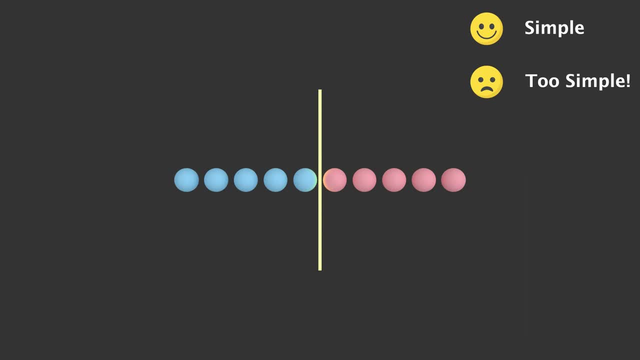 but it is also a limitation, because most datasets in the real world cannot be separated by a hyperplane. A workaround to this limitation is to first apply a non-linear transformation to the data points before applying SVM. With this technique, we can easily achieve the desired. 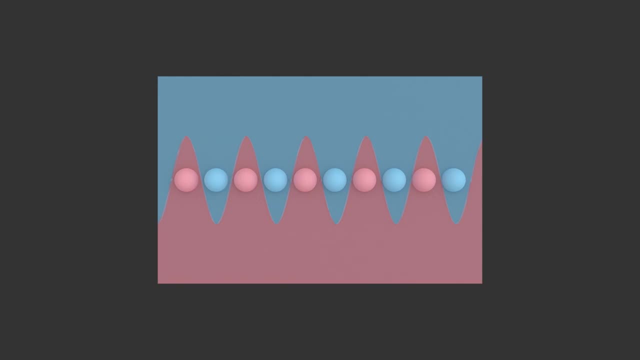 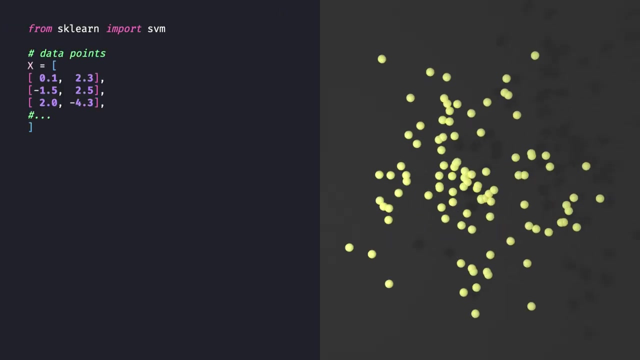 effect of getting a non-linear decision boundary without changing how SVM works internally. This is extremely easy to do. in Python, for example, We load our training data points and labels as usual, but now, when we call SVM's fit function, we don't use x. 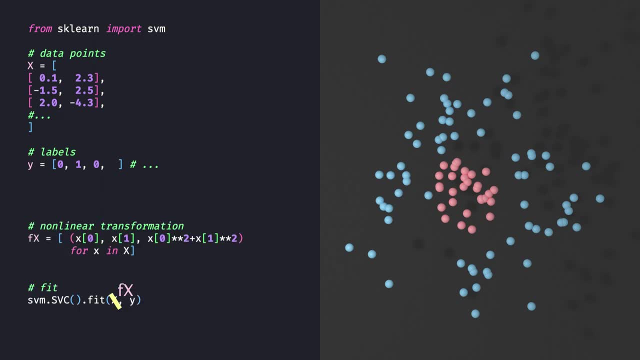 but rather f, where f is a non-linear transformation of x. Geometrically, this non-linear transformation might look something like this: SVM will return a flat hyperplane separating the two classes, as usual, but in the original x space. this coordinate will return a flat hyperplane separating the two classes as usual, but in the 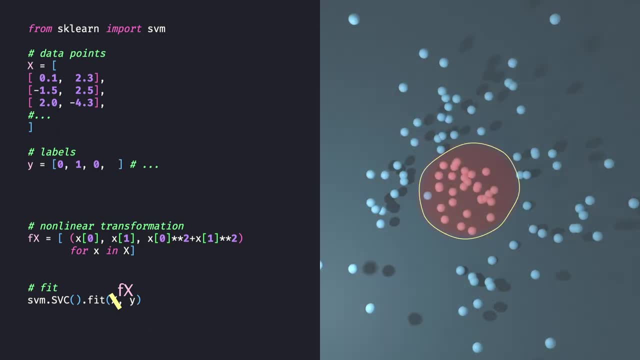 original x space, this coordinate will return a flat hyperplane separating the two classes as usual. but in the original x space, this coordinate will return a flat hyperplane separating the two classes as usual, and this is a non-linear decision. boundary Mission accomplished right. Should we stop here and call it a day? 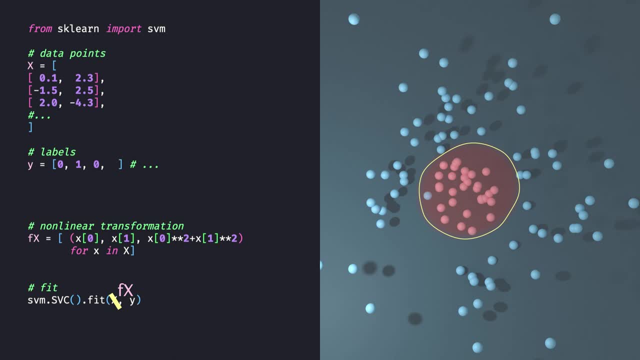 Well, not quite. A first problem is that we need to choose what this non-linear transformation should be. But, as everybody knows, ML enthusiasts are lazy people, so the fewer choices we have to make, the happier we are. The second problem is that if we want a sophisticated decision, boundary 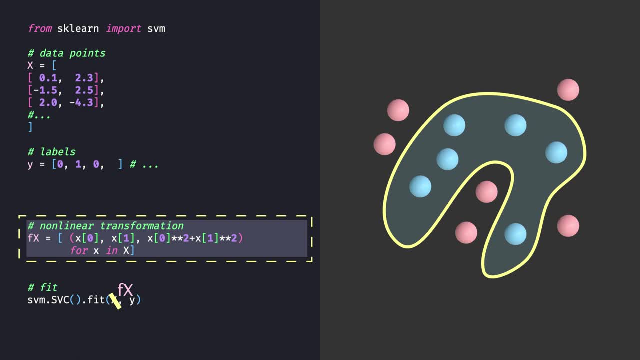 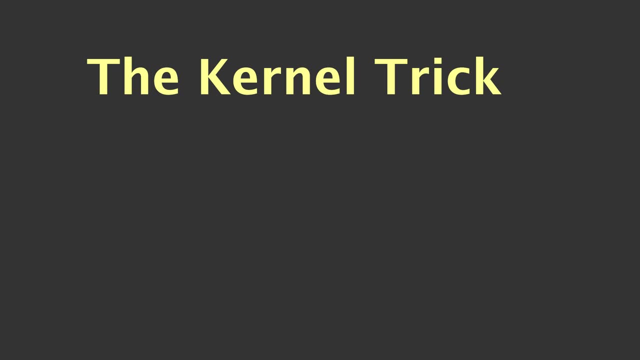 we need to increase the dimension of the output of this transformation, and this in turn increases computational requirements. The so-called kernel trick was invented to solve both of these problems in one shot. The idea is that the algorithm behind this VM does not actually need to know what each 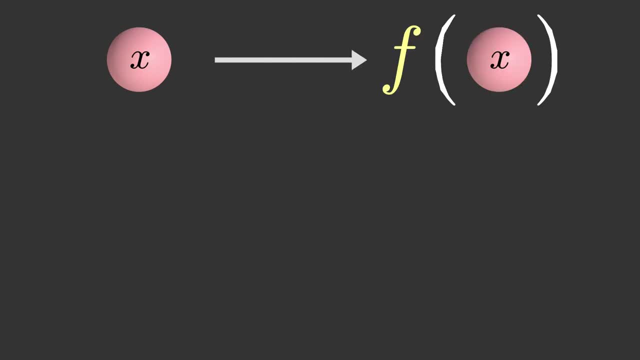 point is mapped to under this non-linear transformation. The only thing that it needs to know is how each point compares to each other. data point after we apply the non-linear transformation. Mathematically this corresponds to taking the inner product between f and f. 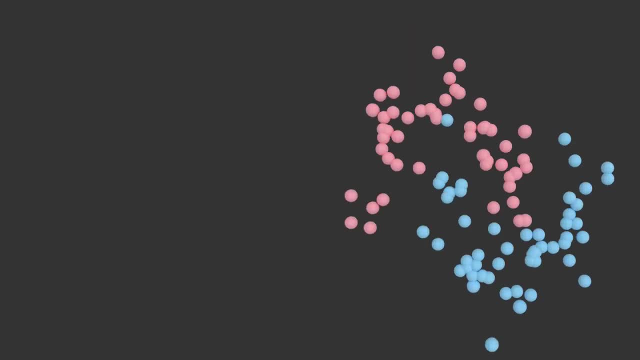 and we call this quantity the kernel function. For example, the identity transformation corresponds to the linear kernel given by x transpose, x, prime. The linear kernel gives a flat decision boundary, which in this case is not good enough to separate the data properly. A polynomial transformation like this one corresponds to the polynomial kernel.